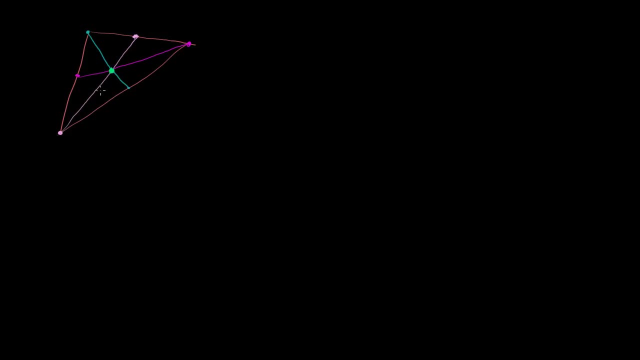 intersect in one point, And that by itself is a pretty neat property, And that one point that they intersect in is called the centroid, And if this was actually a fixed point it would be a physical triangle. Let's say you made it out of iron. 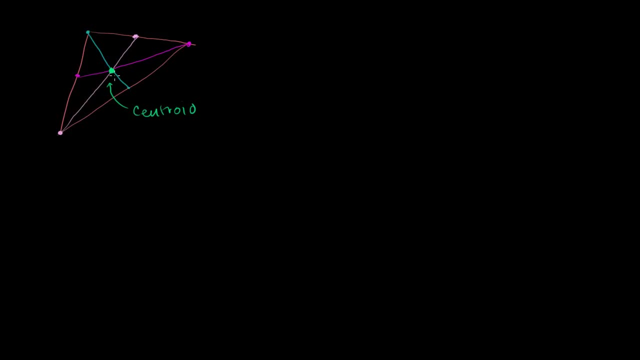 And if you were to toss it, well, even before you toss it, the centroid would actually be the center of mass. So let's say that this is an iron triangle, Let's say that this right here is an iron triangle that has its centroid right over here. 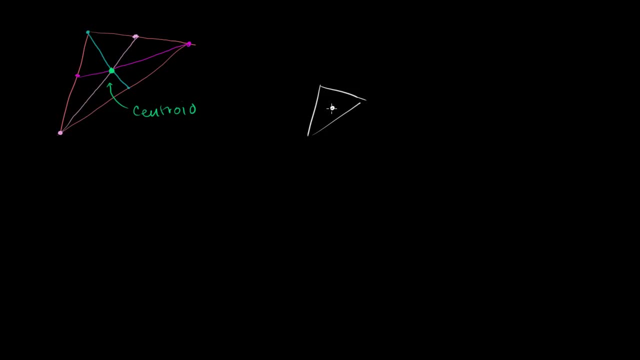 Then this iron triangle's center of mass would be where the centroid is, assuming it has a uniform density. And if you were to throw that iron triangle, it would rotate around this point, Around, Around, Around, Assuming that it had some rotational motion. 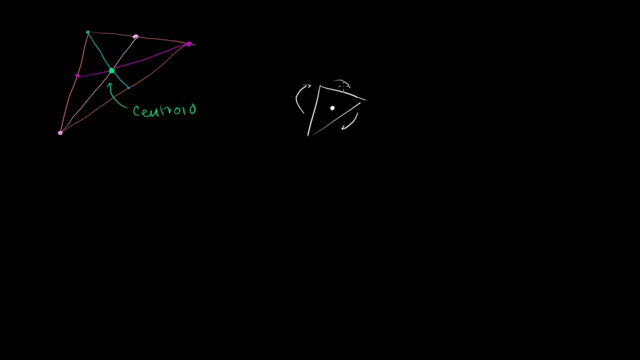 it would rotate around that centroid or around the center of mass. But anyway, the point of this video is not to focus on physics and throwing iron triangles. The point here is I want to show you a neat property of medians, And the property is that if you pick any median, 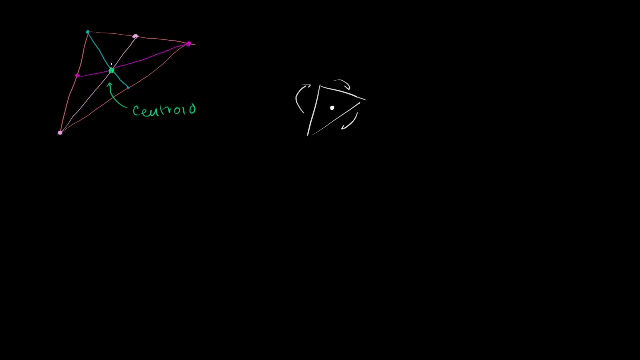 the distance from the centroid to the midpoint of the opposite side. so this distance is going to be half of this distance. So if this distance right here is a, this distance right here is a. So if this distance right here is a, this distance right here is a. 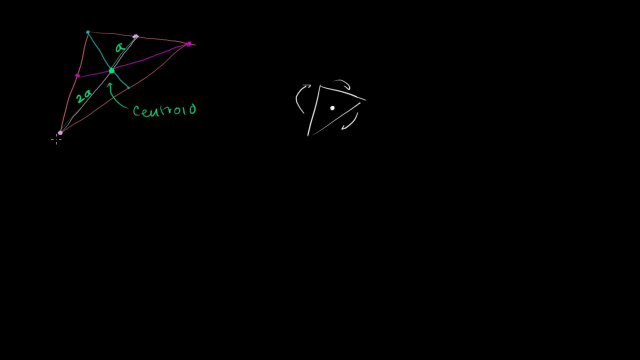 So if this distance right here is a, this distance right here is a, Then this distance right here is 2a. Or another way to think about it is: this distance is 2 thirds of the length of the entire median And this distance right here is 1 third. 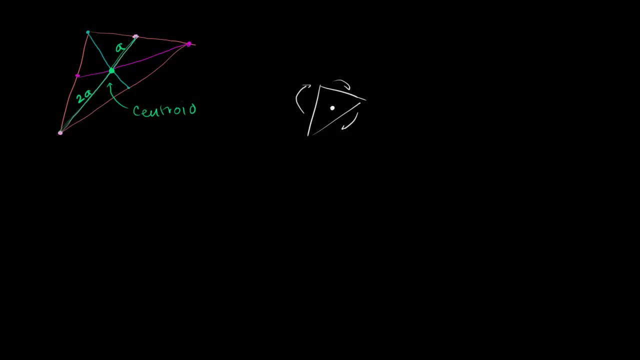 of the length of the entire median. And let's just prove it for ourselves, just so you don't have to take things on faith. And to do that, I'll draw an arbitrary triangle, I'll do a two-dimensional triangle And I'll do it in three dimensions. 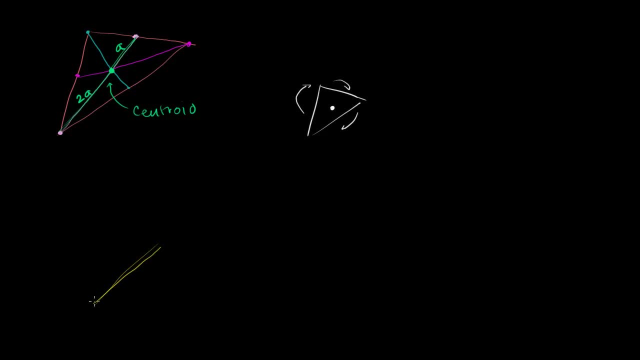 because, at least in my mind, it makes the math a little bit easier. In general, whenever you take a, let's say In general, whenever you take a, whenever you have an n-dimensional figure and you embed it in n plus 1 dimensions, 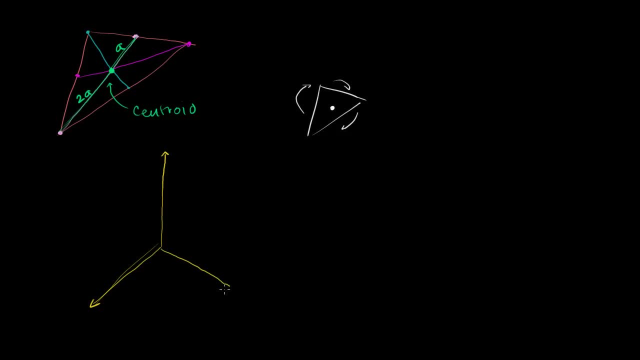 it makes the math a little bit easier. The actual tetrahedron problem that we did. you could actually embed it in four dimensions and it would make the math easier. It's just much harder to visualize, So I didn't do it that way. 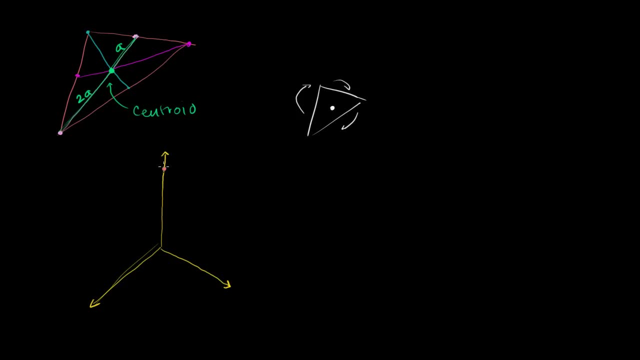 But let's just have an arbitrary triangle And so let's say it has a vertex there, a vertex there and a vertex there. So I'm not making any assumptions about the triangle. I'm not saying it's isosceles or equilateral or anything. 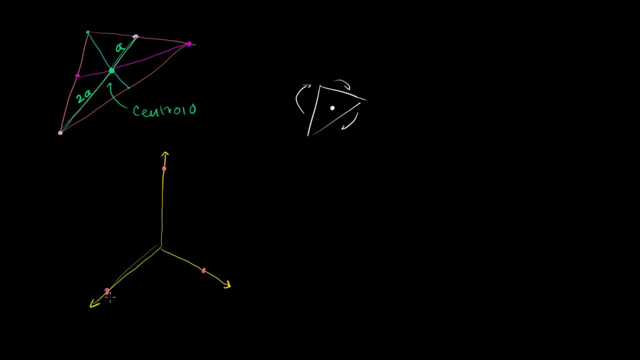 It's just an arbitrary triangle, And so let's say its coordinate. let's say this coordinate right over here is, I'll call this, the x-axis. So this is the x-axis, the y-axis and the z-axis. I know some of y'all are used to swapping these two axes. 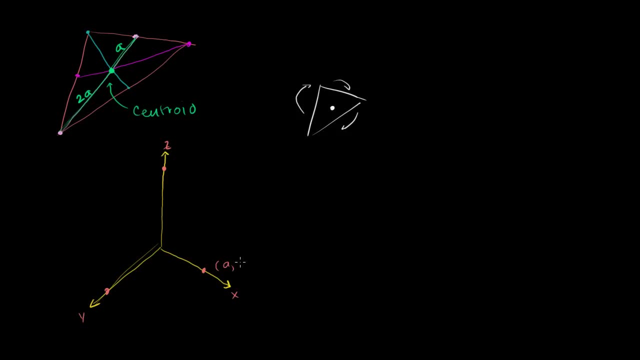 But it doesn't make a difference. So let's call this coordinate right here a 0, 0.. So it's a along the x-axis. Let's call this coordinate 0, b 0.. And let's call this coordinate up here 0, 0, 0,, 0, 0.. 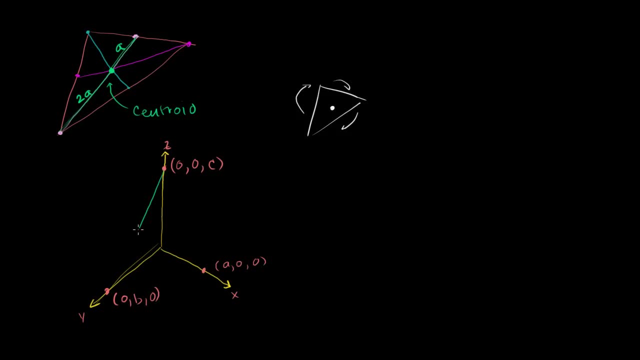 So see, if you connect the points, you're going to have a triangle. You're going to have a triangle, just like that. Now, the centroid of a triangle, especially in three dimensions, the centroid of a triangle is just going to be the average of the coordinates of the vertices. 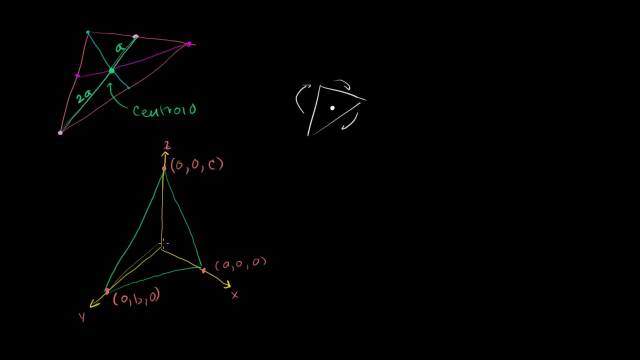 or the coordinate of the centroid. The coordinate of the centroid here is just going to be the average of the coordinates of the vertices, So this coordinate right over here is going to be. so for the x-coordinate we have 0, plus 0, plus a. 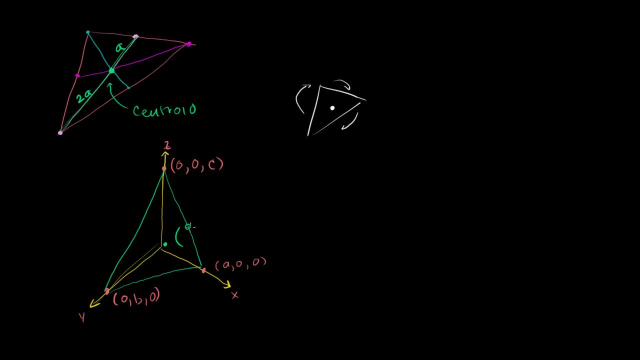 So we have three coordinates. They add up to a and we have to divide by 3. So it's a over 3.. The y-coordinate is going to be b plus 0, plus 0.. They add up to b, but we have three of them. 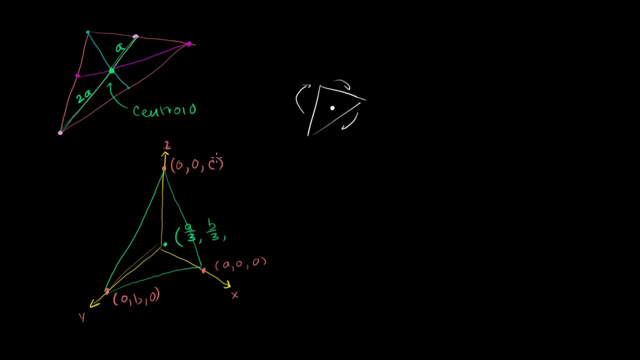 So the average is b over 3.. And then same thing, we do it for the z-coordinate. The average is going to be c is c over 3.. And I'm not proving it to you right here. You could verify it for yourself that it's. 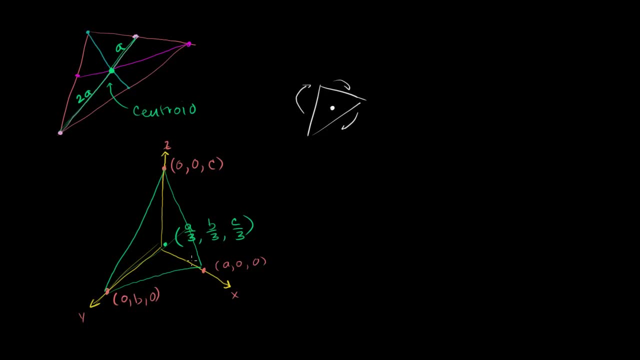 going to be the average. that, if you were to figure out what this line is, this line is and this line is this centroid or the center of mass of this triangle, if it had some mass, is just the average of these coordinates. 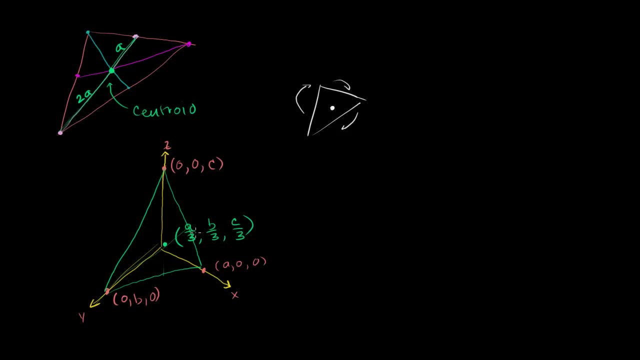 Now what we want to do is use this information. Let's just use this coordinate right here and then compare, just using the distance formula. let's compare this distance up here in orange to this distance down here in yellow, And remember this point right over. here is the point. 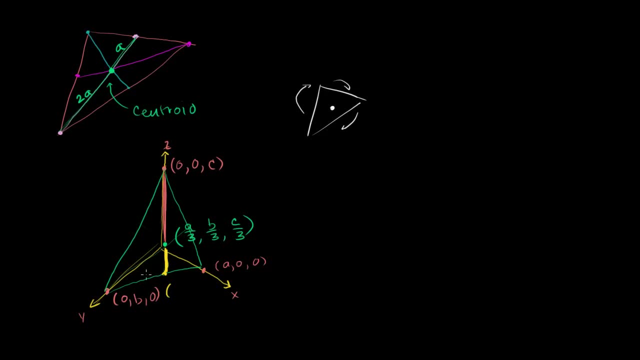 this is the median of this bottom side right over here. So the median of that bottom side is just going to be the average of these two points, And so the x-coordinate- 0 plus a over 2, is going to be a over 2.. 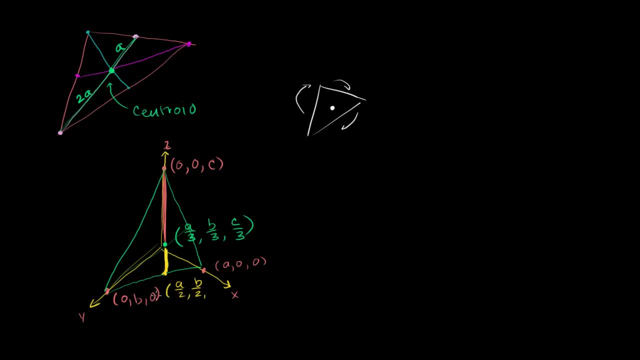 b plus 0 over 2 is going to be b over 2.. And then it has no z-coordinate, so it's just going to be 0.. 0 plus 0 over 2 is 0. So we know the coordinates for this point. that point. 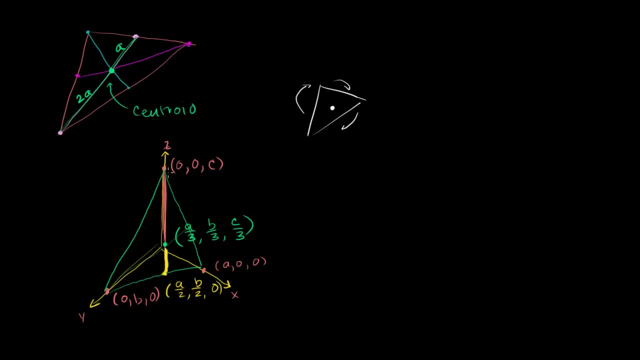 and that point. so we can calculate the yellow distance and we can calculate the orange distance. So let's calculate the orange distance. So that is going to be equal to the square root. the orange distance is going to be equal to the square root of. 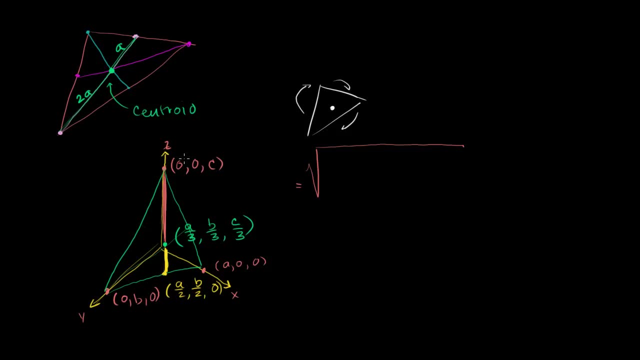 and we just take the difference of each of these points squared, So it's a over 3 minus 0 squared, So that's going to be a squared over 9, plus b over 3 minus 0 squared, So that's b squared over 9, plus c over 3. 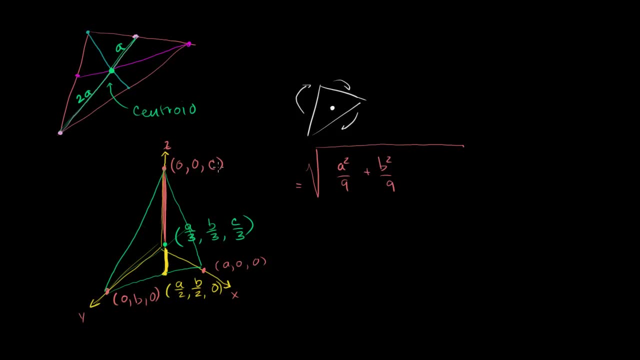 minus c, which is negative 2 thirds. That's negative 2 thirds and we want to square that. So we're going to have positive 4 over 9 c squared. Did I do that right? c over 3, so 1 third minus 1 is negative 2 thirds. 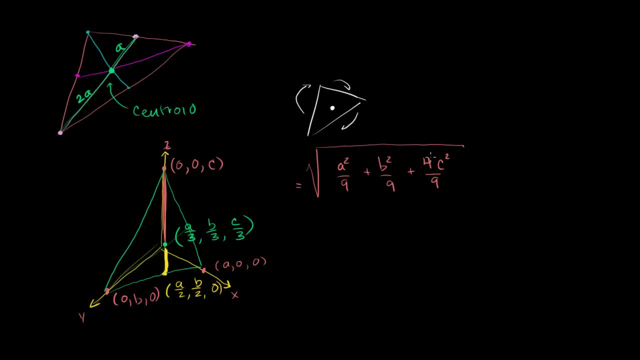 So this is negative, 2 thirds c. You square it, you're going to get 4, 9 c squared. So that's the orange distance. Now let's calculate, and if we want to do it, we can actually express this: 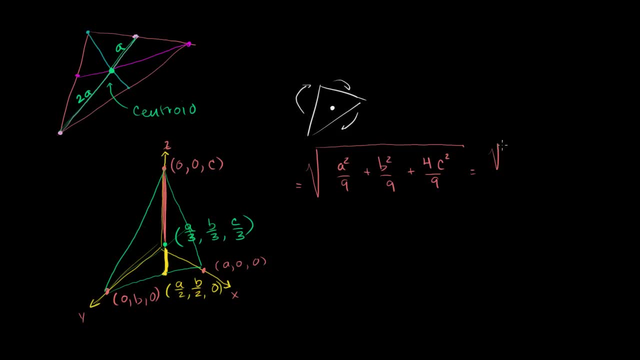 Let me express it a little bit simpler than this. This is the same thing as the square root of a squared plus b squared plus 4, c squared over the square root of 9, which is just equal to 3.. Now let's do the same thing with the yellow distance. 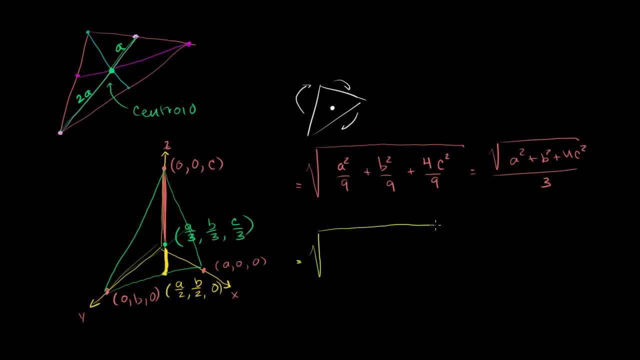 So it's going to be equal to the square root of. so if we have a over 2 minus a over 3, so 1 half minus 1 third, that's the same thing as 3, 6 minus 2, 6, so it's 1: 6 a.